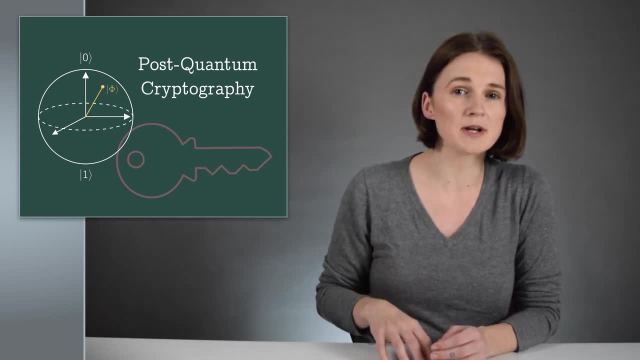 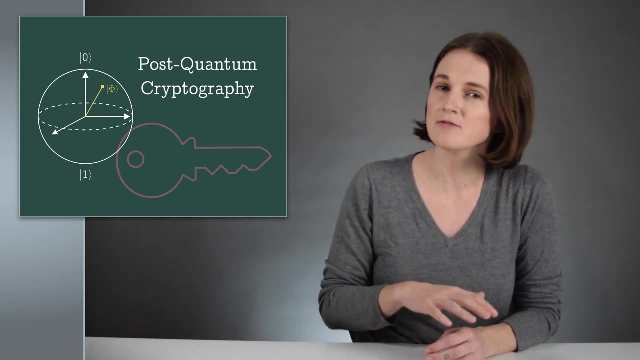 is designed to defend against this. It's about creating cryptographic algorithms which are secure against attacks from a quantum computer. Many of the most promising algorithms are designed to defend against this. It's about creating cryptographic algorithms which are secure against attacks from a quantum computer. Many of the most promising algorithms are 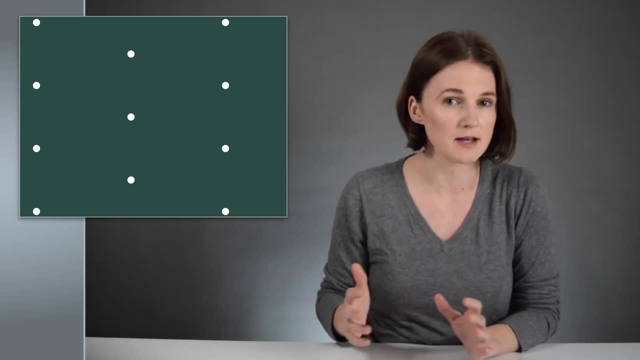 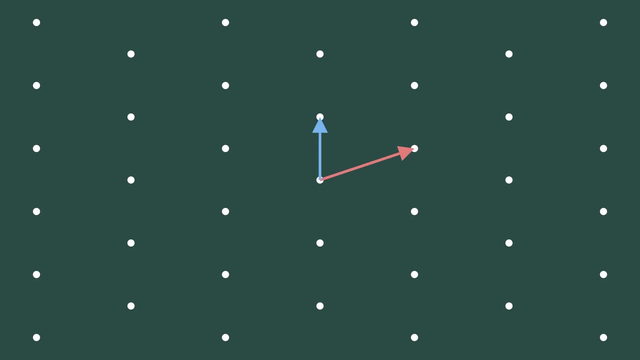 lattice-based meaning. they have something to do with these kinds of pictures. More precisely, this two-dimensional lattice is generated or created by these two vectors or arrows. We start with a dot at the origin and dots at the end of each basis vector. From there, 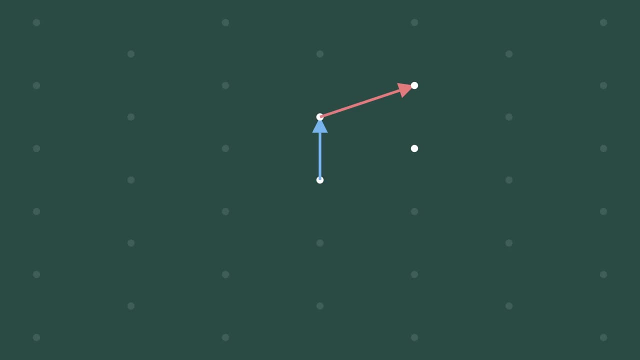 we build, We lay down the vectors like dominoes to form paths starting from the origin, And the lattice is made up of all of the points that we can reach with these vector snakes. For example, this point is two times the red vector plus one times the blue vector. 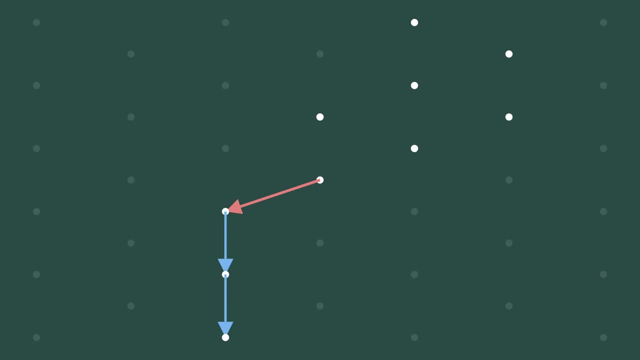 The vectors can be flipped around and we can stack any number of them together. We could describe this point as negative one red plus negative two blue plus one red, but we can lump the reds together and then they'll cross each other out. 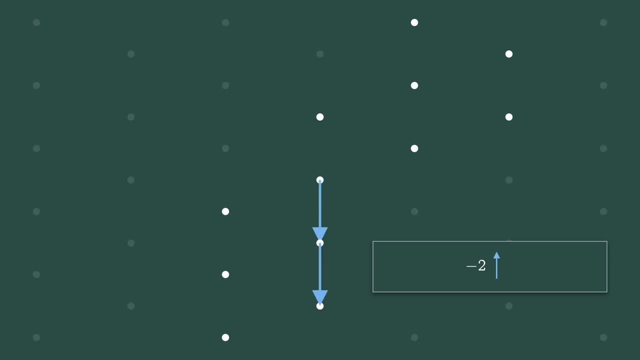 So it's really just negative. two blue- The blue and the red vectors are a basis for this lattice. They're used to build all the points. As the basis vectors move, so do the lattice points. Let's look at this on the usual two-dimensional plane. Say that our basis vectors are one zero in. 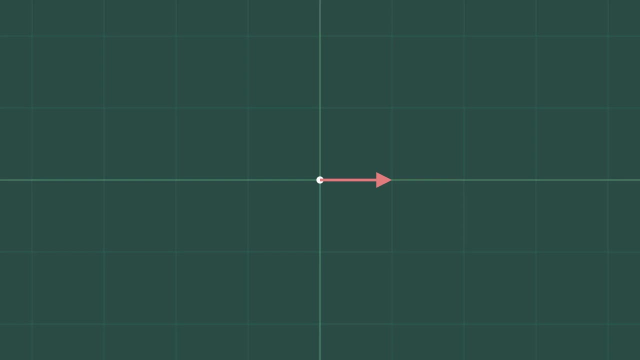 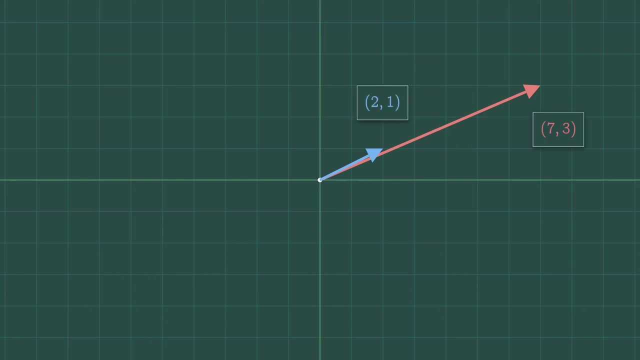 red, one in the x-direction and zero in the y-direction and zero one in blue. These make the normal square lattice. But zooming out, what if we use these two basis vectors, seven, three and two one? The coordinates of our basis vectors will always be whole numbers. 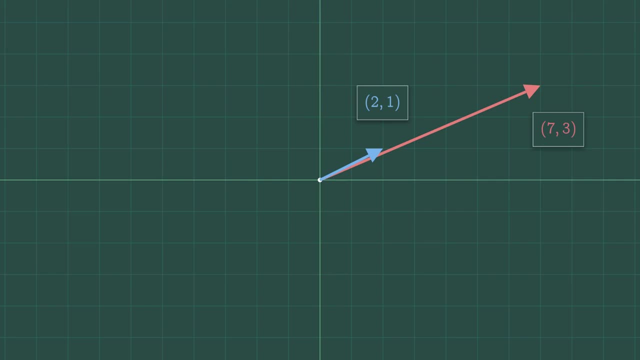 Let's start by constructing some lattice points by putting dots at the ends of the vectors. We can add two blue vectors or just one negative red vector or one negative blue vector. At first they look to be creating points on a line, but if we start stacking together positive 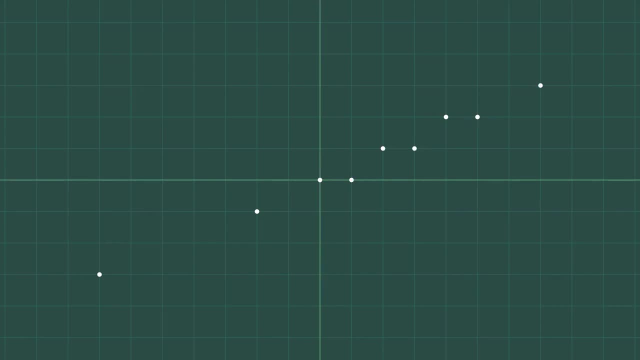 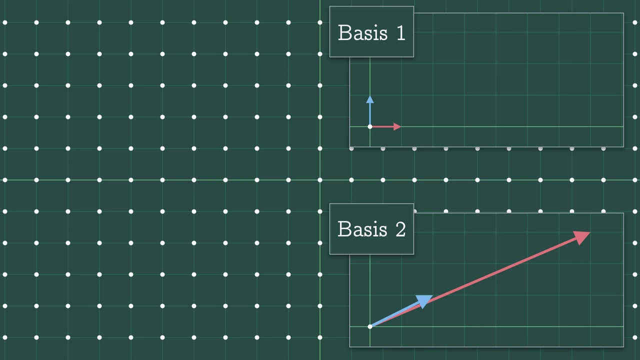 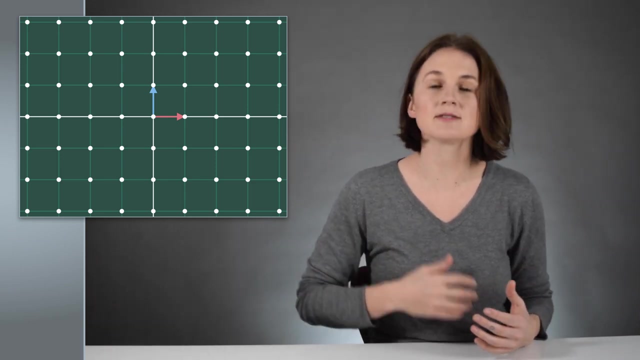 and negative vectors, we get other points and eventually you'll end up with the same square lattice. This illustrates an important point: Two very different looking sets of basis vectors can generate the same lattice. That lattice was pretty easy to describe. It's all the points. 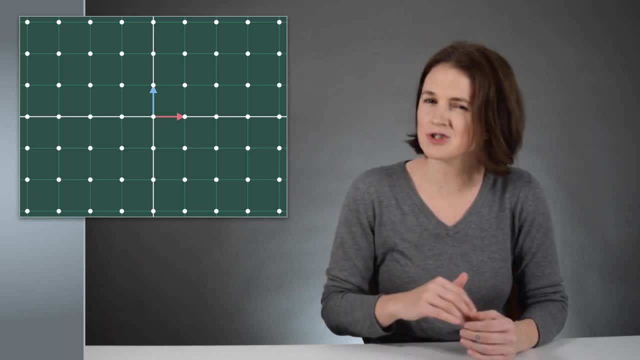 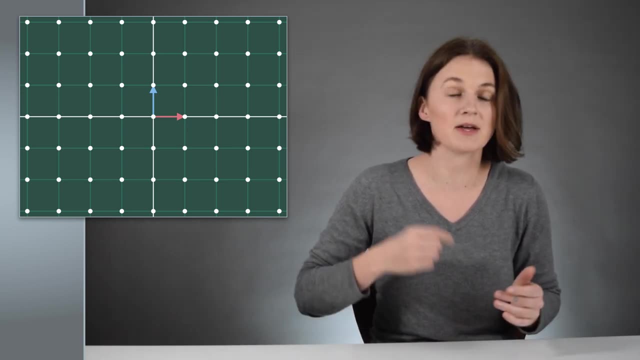 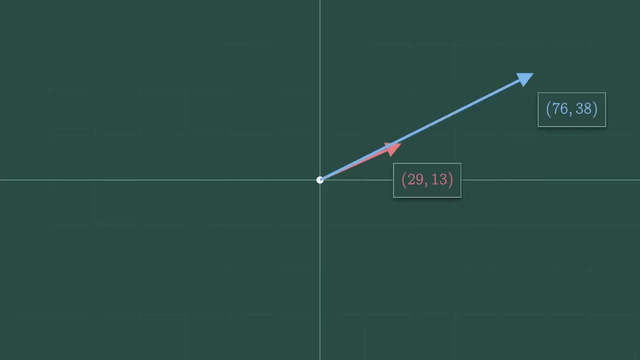 with integer or whole number coordinates, But in general it's not so easy to do that, to describe all the points on a lattice, except to say it's the lattice generated by these vectors. For example, here are two other basis vectors: 29,, 13, and 76, 38. What does the lattice generated? 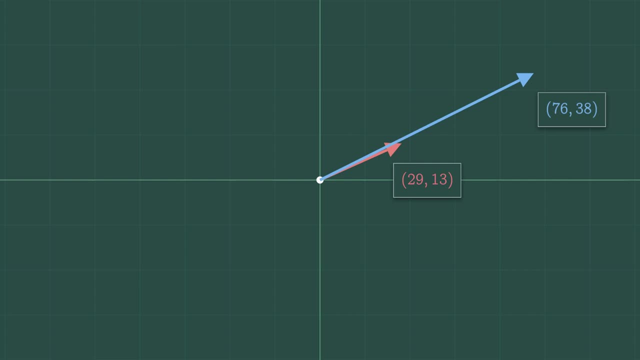 by these vectors look like We can start to fill in some points, starting with the two points at the ends of the basis vectors. We can add them together to get a hundred and five fifty one but 1, or take red minus blue to get negative 47, negative 25.. 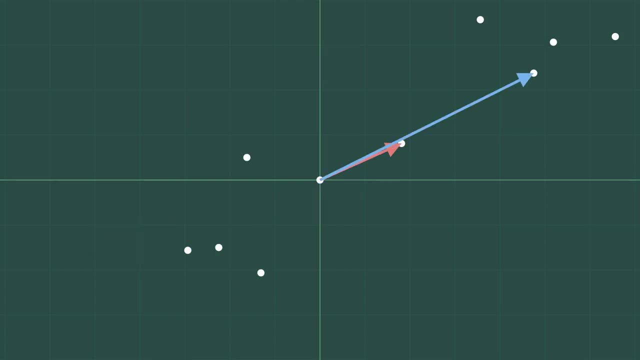 We can start building up individual points, but the full picture isn't necessarily obvious. Here's a surprisingly hard question: Which point on the lattice is closest to the origin? 0, 0, not including the lattice point that is at the origin. 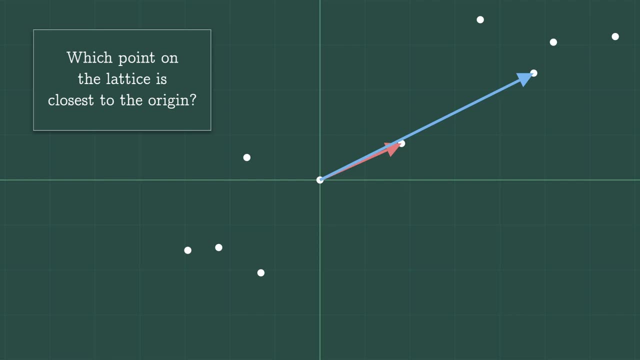 Here's another way to think about it: Which combination of the vectors is closest to 0, 0?? For example, 3 reds minus 1 blue vector gives us 11, 1.. That's pretty close, but can we do better? 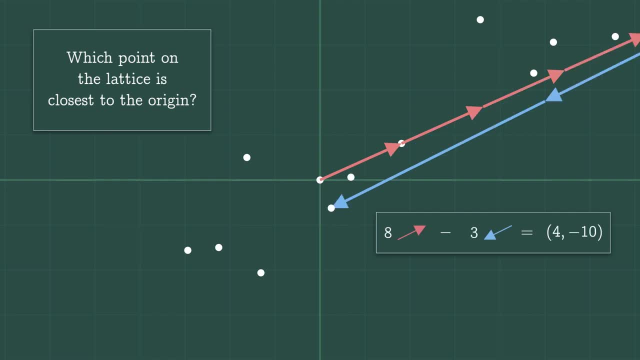 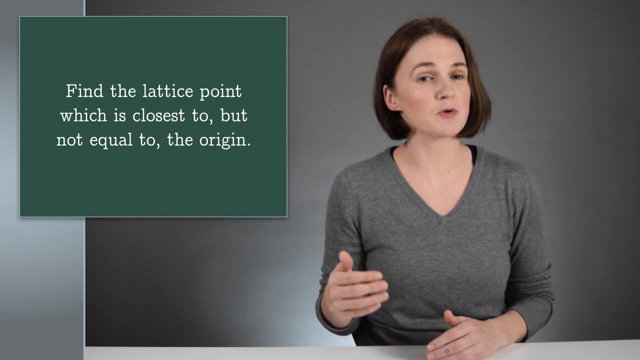 Yes. For example, 8 red minus 3 blue vectors is 4, negative 10,, which is slightly closer to the origin. This problem find the lattice point which is closest to but not equal to the origin, is called the shortest vector. 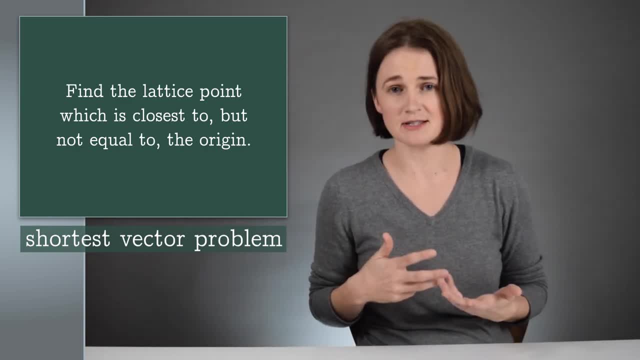 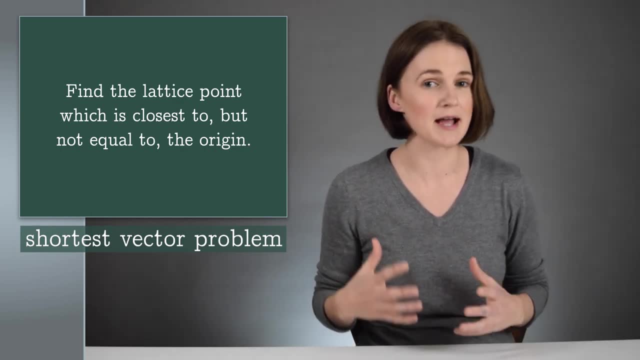 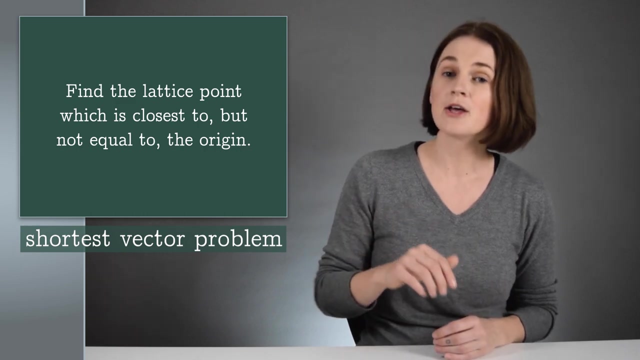 problem. Our method, trying different combinations that seemed good, was pretty inefficient. It's possible that the Optimal solution comes from adding together many red and blue vectors In two dimensions. you could probably reason your way to a solution. But the shortest vector problem gets very hard in higher dimensions. 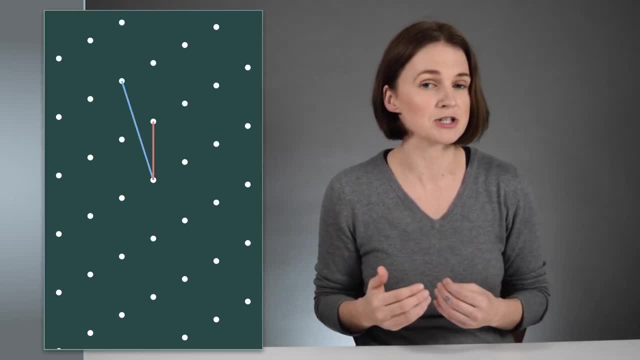 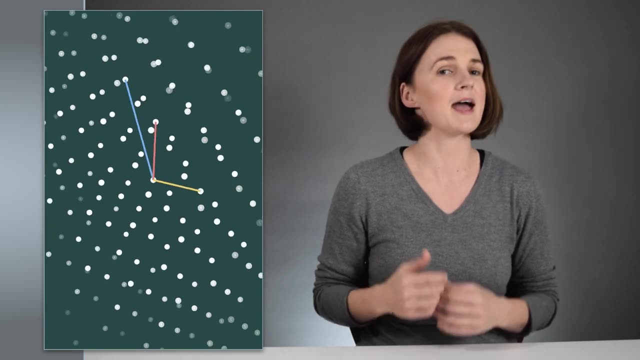 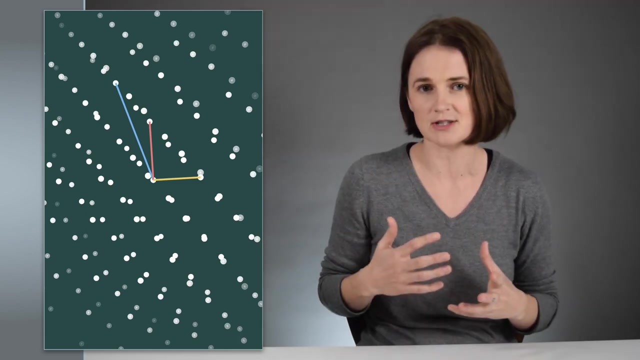 We used two basis vectors with two coordinates to create a two-dimensional lattice. But if we had used three basis vectors with three coordinates, we would get a three-dimensional lattice, And 17 basis vectors gives you a 17-dimensional lattice. There's more possibilities in higher dimensions. 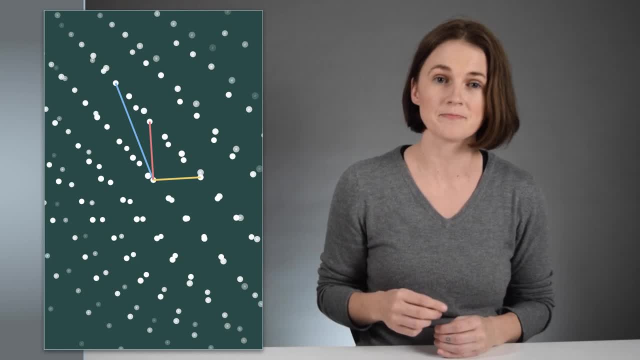 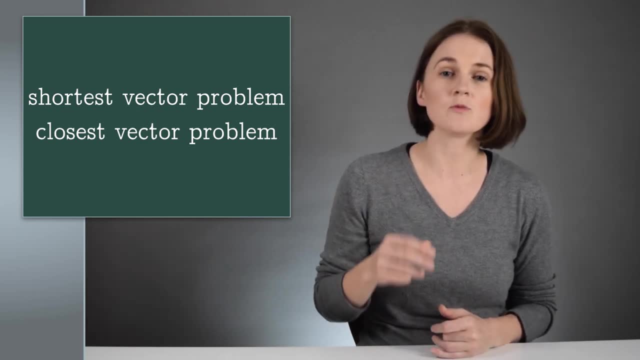 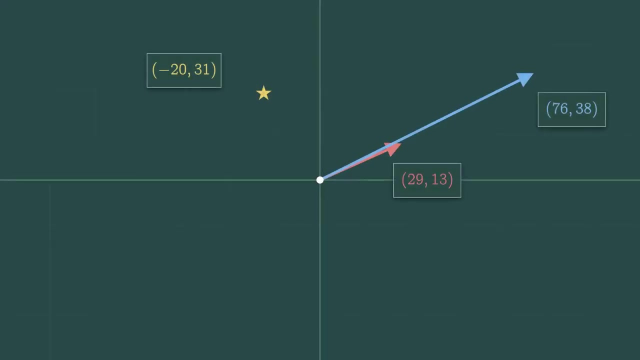 and the shortest vector problem is even harder. The shortest vector problem is similar to the closest vector problem. Find the lattice point which is closest to a particular point in space. For example, which point on the lattice generated by the two vectors from before is closest to negative? 20,, 30,, 1?? 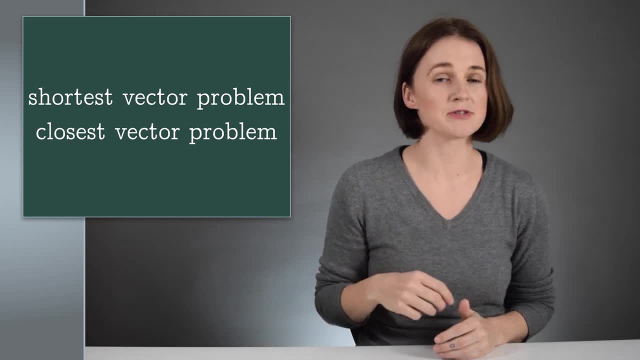 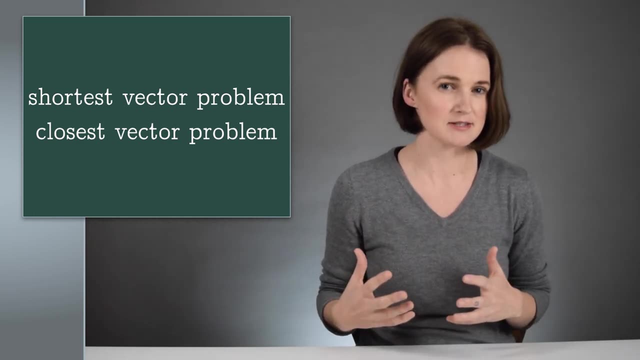 These belong to a collection of related problems known as lattice problems. So let's take a look at one example: problems which experts believe to be hard problems, especially in hundreds of dimensions. In other words, it would generally take a computer a very long time to solve the shortest. 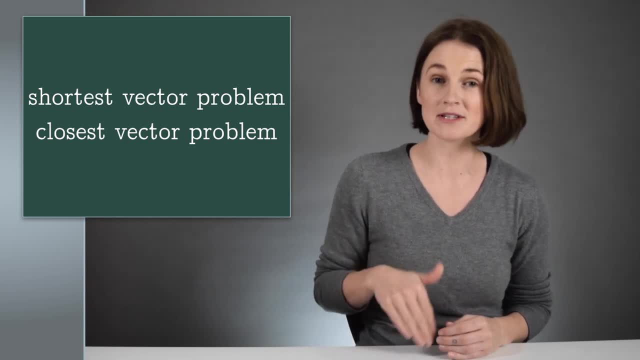 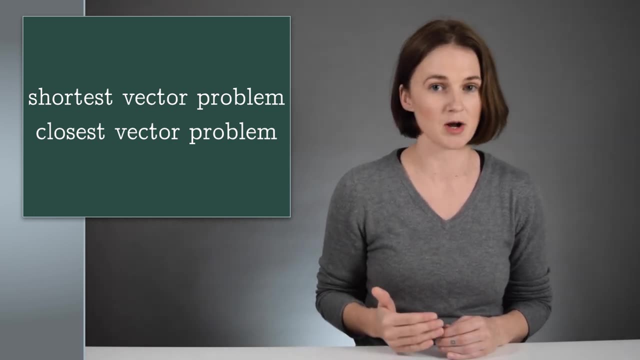 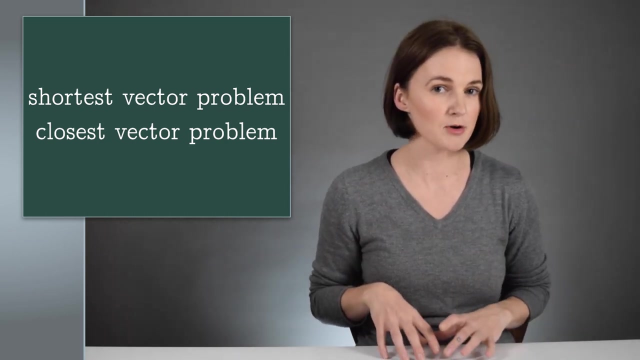 or closest vector problems And, importantly, for our purposes. computer scientists also believe that it would be very difficult for a quantum computer to solve these problems. That makes them good candidates for the mathematical basis for a quantum secure cryptographic protocol. How would that work? 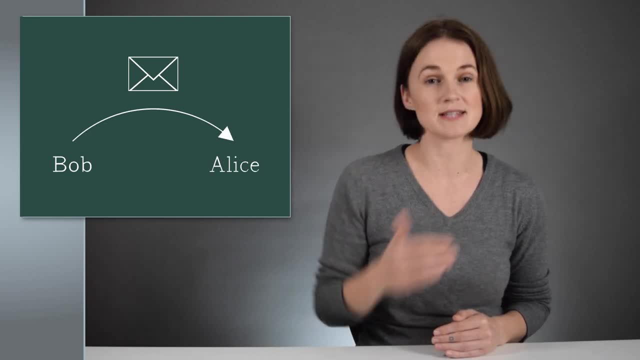 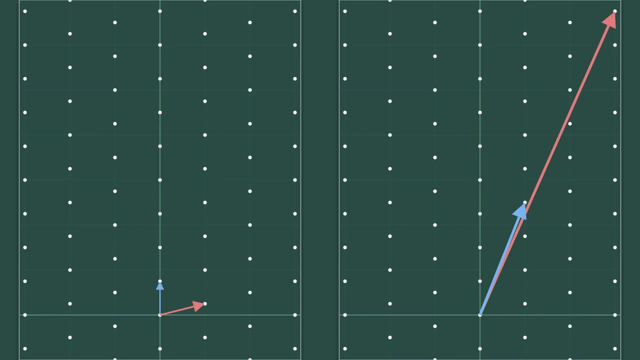 Well, here's one idea. Let's say Bob wants to send Alice a message. First, Alice sets up a lattice with two different bases. In other words, both bases generate the same lattice. In one basis the vectors are close to perpendicular. 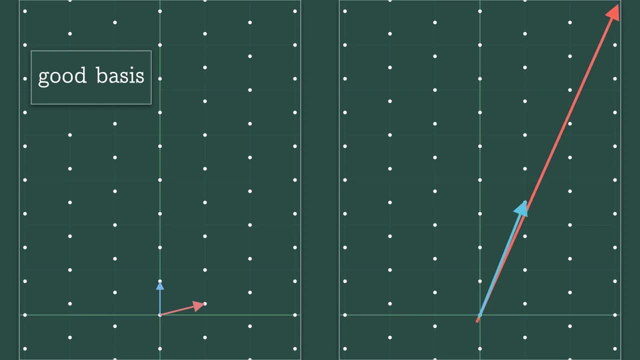 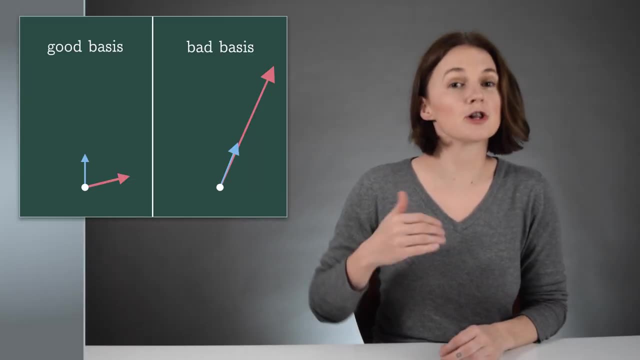 We're going to call that a good basis. In the other basis the vectors are much closer to parallel. We're going to call that a bad basis. Here's a fact: The closest vector problem is much harder to solve. It's much harder to solve with a bad basis than a good basis. 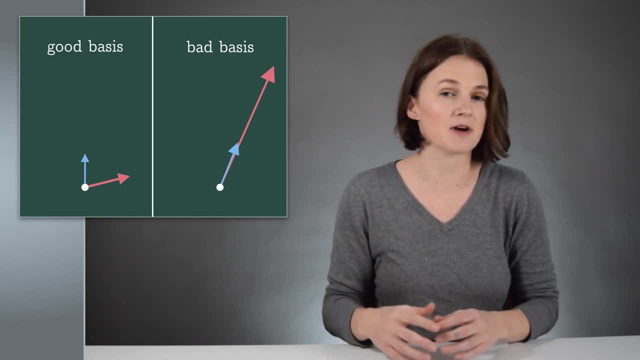 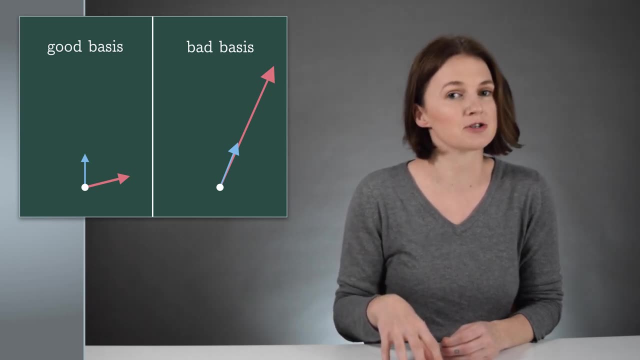 If you know a good basis for the lattice it can be somewhat easy to find the closest lattice point. But if you only know a bad basis for the same lattice, it can be much harder to solve the same problem. The bad basis vectors are almost in a line. 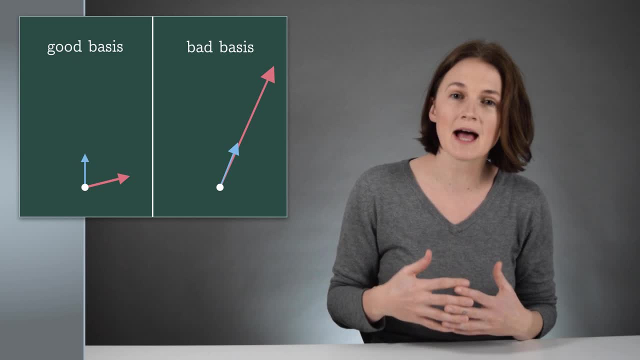 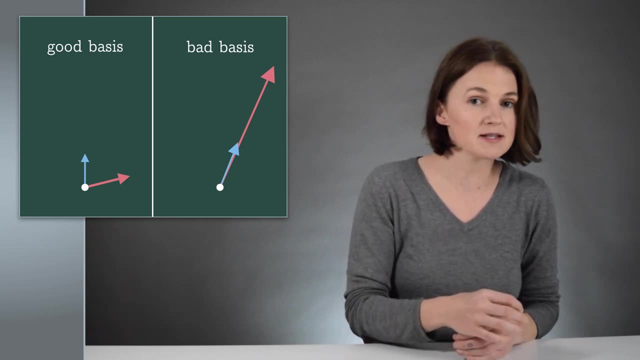 They can nearly cancel each other out. So the closest lattice point may come from adding and subtracting many, many vectors. So Alice keeps the good basis a secret. So Alice keeps the good basis a secret. So Alice keeps the good basis a secret. 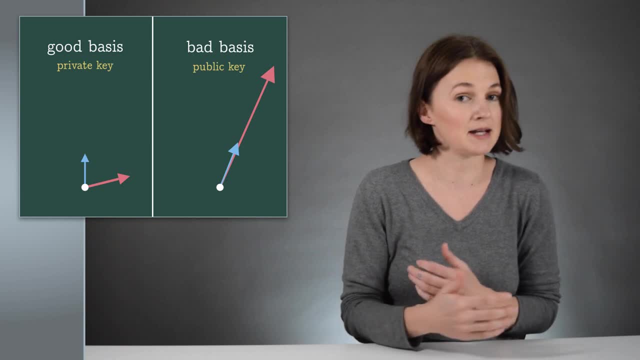 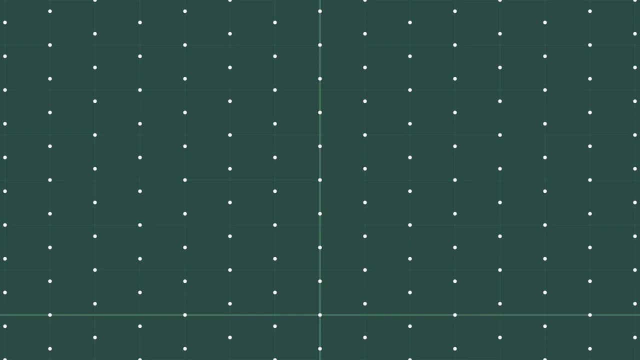 That's private information, But she tells Bob and anyone else who might be eavesdropping the bad basis. Now Bob uses that basis and embeds a message in the lattice. He picks a point on the lattice, the yellow one, which somehow represents his message.